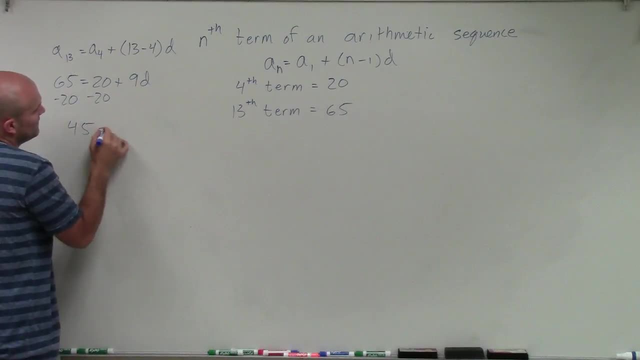 d. So I subtract 20, and therefore I get 45 equals 9d. Divide by 9,, divide by 9, that's a d, And we can say d equals 5.. So now I know the common difference right. However, there's 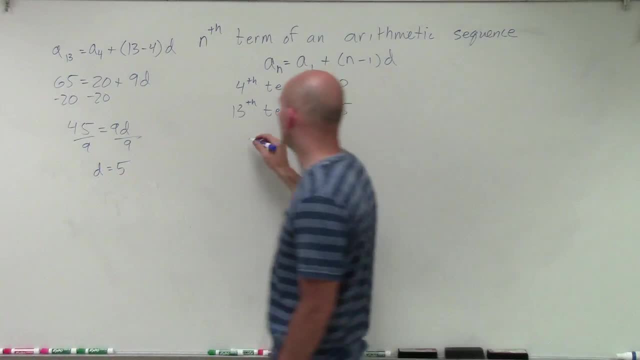 a little bit of a problem, because to write this formula, if I want to find the formula, it needs to be: a sub n equals a sub 1.. So I need to figure out what is my a sub 1.. Now we can do this. 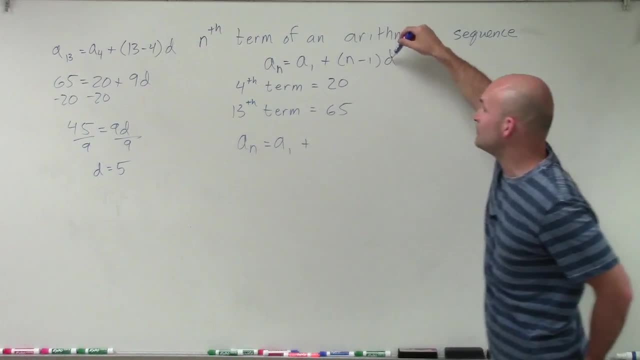 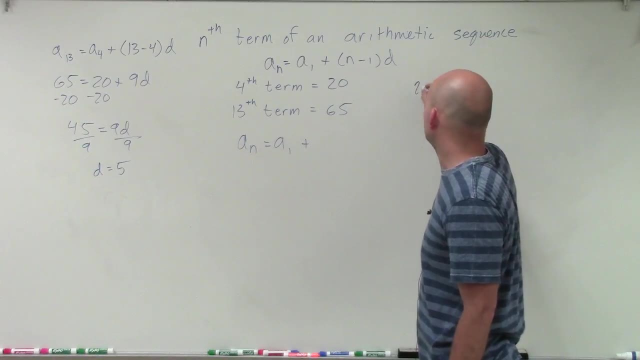 exact same process again. This time, now that we know d, we could say, all right, I need to figure out. let's say, I know a sub 4.. So I know a sub 4, which would be 20. So I could. 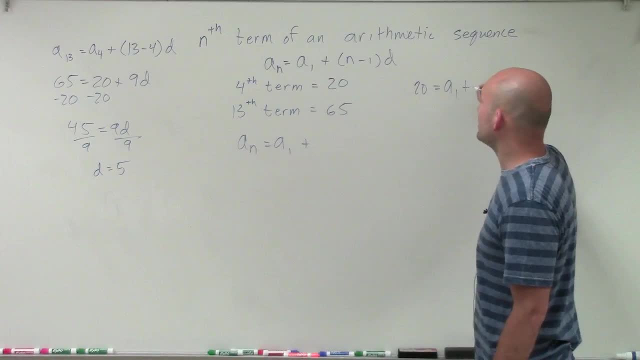 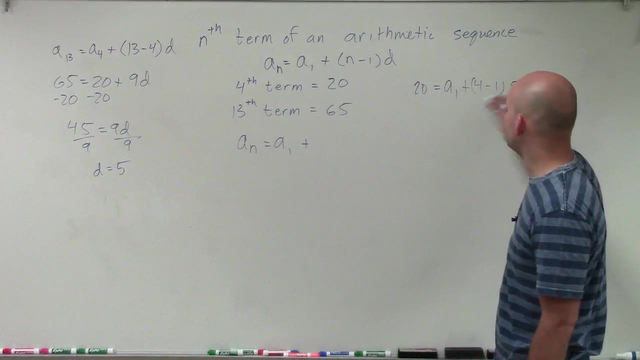 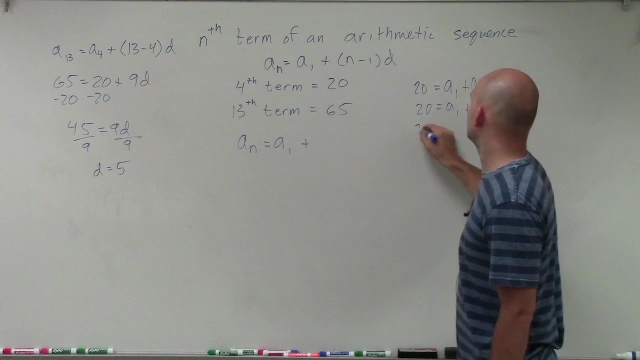 say 20 equals- I do not know what a sub 1 is- plus 4 minus 1 times my difference, which is 5, right? And you could say: 20 equals a sub 1.. 20 equals a sub 1 plus 3 times 5.. 20 equals a sub 1 plus 15, minus 15.. And you could say: 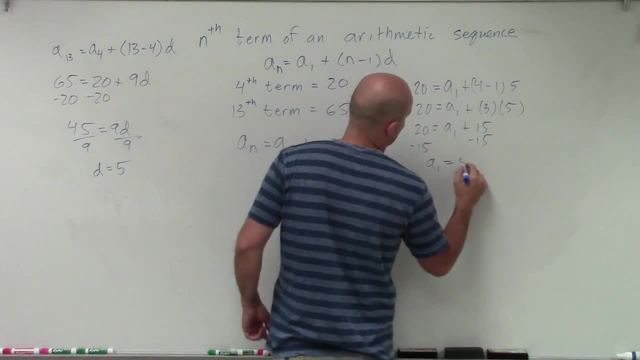 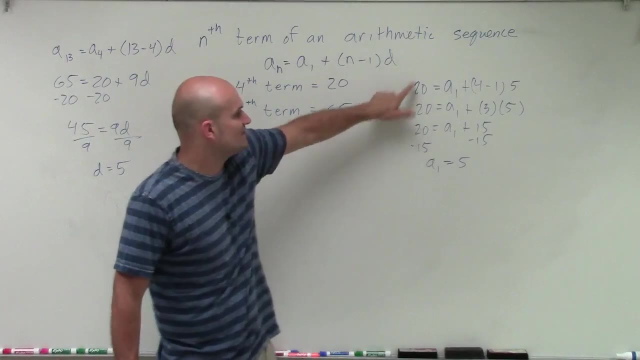 a sub 1 equals 5,. right, So you can follow that process. You could do the same thing for the 13th term instead of using the 13th term, or you 65 here and 13 over there. However, 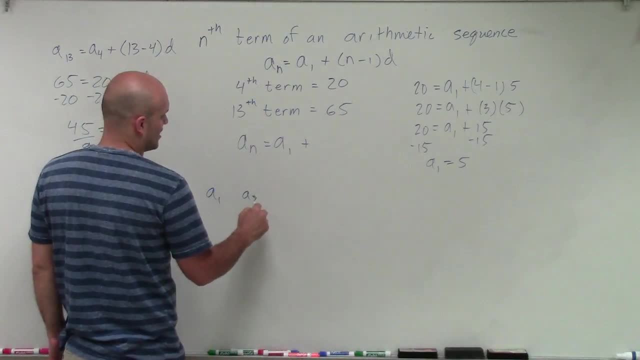 we could also just kind of look at this and just say, all right, well, if I know a sub 1, a sub 2, a sub 3, a sub 4,, well, if a sub 4 is 20, and I know the difference between. a sub 2 and a sub 3,, I know that's a sub 2, so I can say a sub 4 is 5.. If I know a sub 2 is 5,, I know that's a sub 4,. and if I know a sub 4 is 5,, I know that's a sub 4, and if I 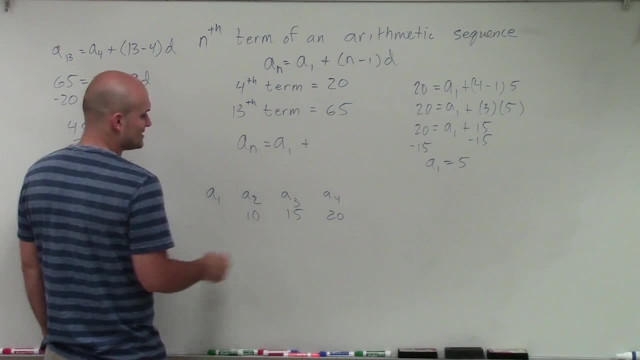 difference is 5, then a sub 3 has to be 15,, a sub 2 has to be 10, and a sub 1 equals 5.. So you can really kind of work at it either way. But the main important thing though. 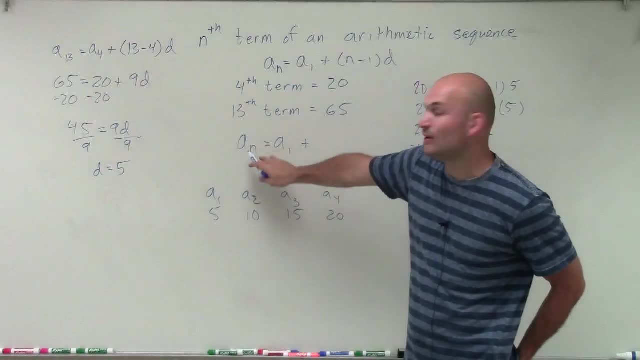 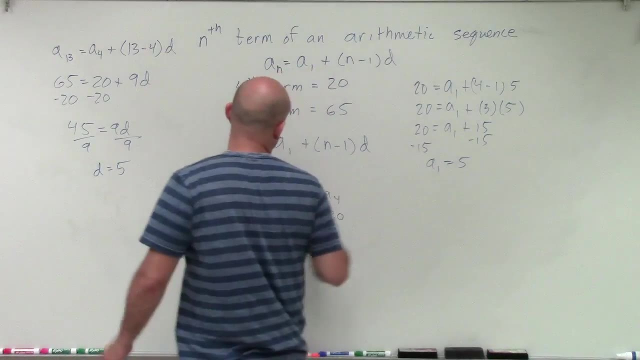 is. now we know what a sub 1 is and we want to find the equation for any value of a sub n. So it's going to be plus at minus 1, and then now our difference now is d. Well, now we know what d is and we know what a sub 1 is. So let me write this in a different